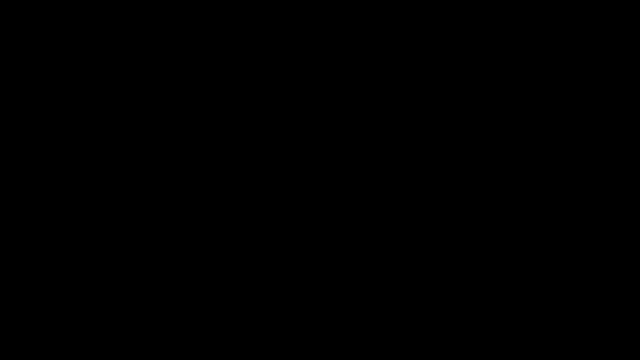 I want to do a quick video on something that you're likely to see in a statistics class, and that's the notion of a type one error, And all this error means is that you've rejected. this is the error of rejecting. let me do this in a different color: rejecting the null hypothesis, even though it is true. 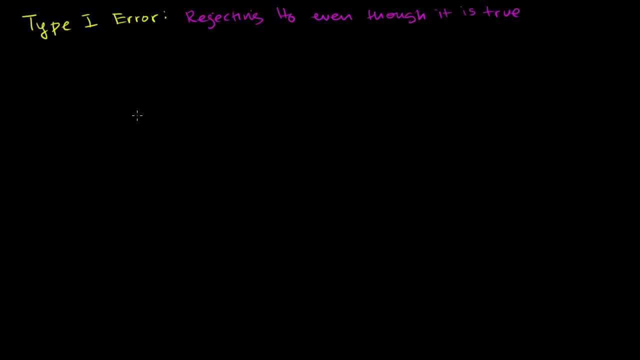 It is true. So, for example, in a lot of the, in actually all of the hypothesis testing examples we've seen, we start assuming that the null hypothesis is true. We assume, we always assume- that the null hypothesis is true And, given that the null hypothesis is true, we say okay, if the null hypothesis is true. 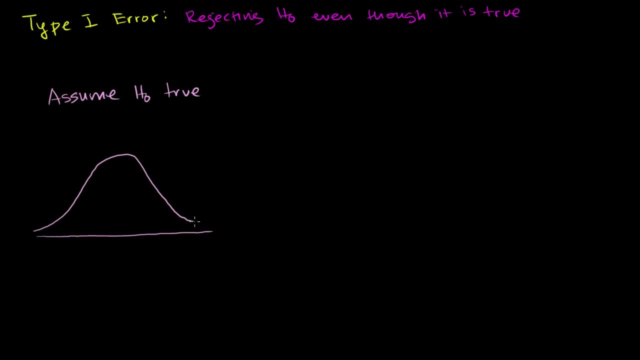 then the mean is usually going to be equal to some value. So we create some distribution, assuming that the null hypothesis is true, It normally has, it has some mean value right over there. And then we have some stat, we have some statistic. 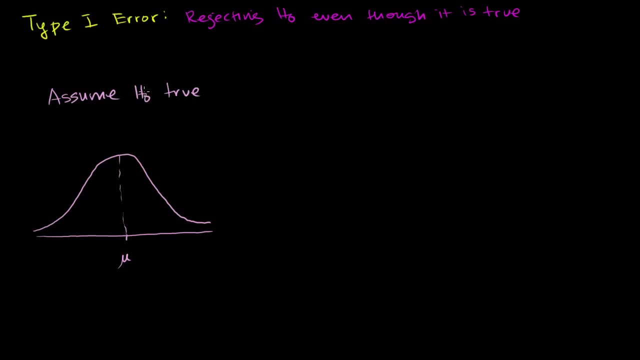 We have some statistic and we are seeing if the null hypothesis is true, what is the probability of getting that statistic Or or getting a result that extreme or more extreme than that, that statistic? So let's say that the statistic gives us some value over here. 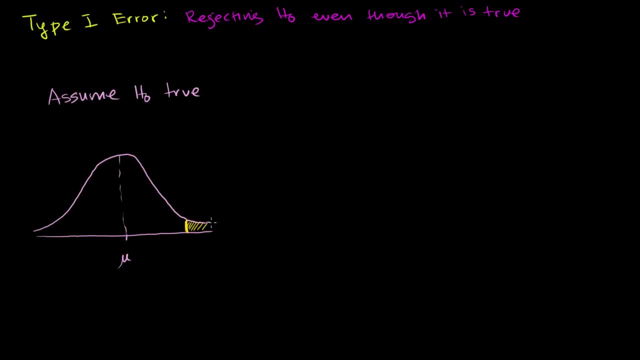 And we say, gee, you know what? There's only a, there's only- I don't know- there might be a 1% chance. There's only a 1% chance. There's only a 1% probability. there's only a 1% probability of getting a result that 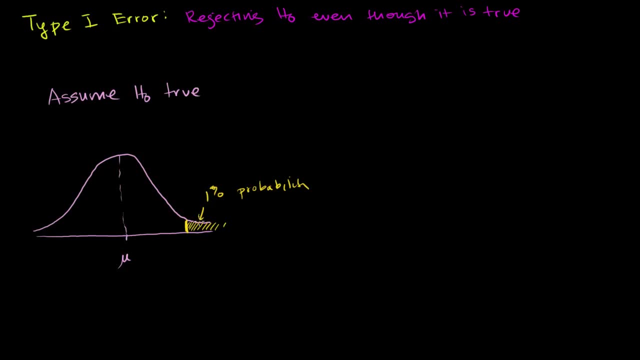 that extreme or greater. And then, if, if that's, I guess, low enough of a threshold for us, we will reject, we will reject the null hypothesis. So in this case, in this case, we will. So let's say, let's say that, actually, let's think of it this way: 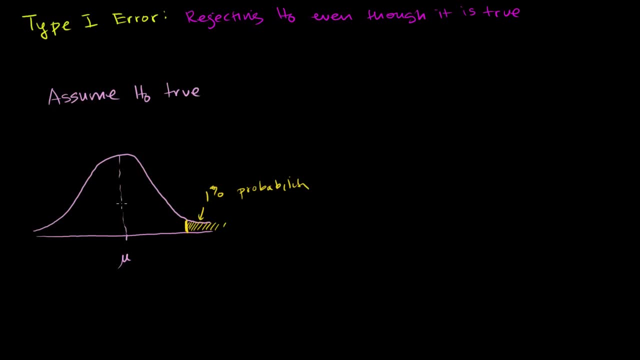 Let's say that 1% is our threshold, We say, look, we're going to assume that the null hypothesis is true. There's some threshold That if we get, if we get a value any more extreme than that value, there's less than. 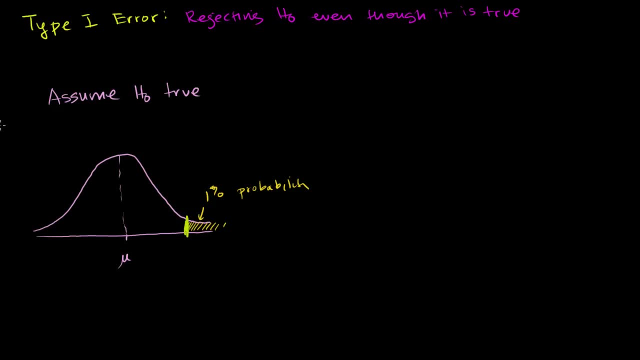 a 1% chance of that happening. So let's say we're looking at sample means and we get a sample mean that is way out. here We say, well, there's less than a 1% chance of that happening. given that the, given that